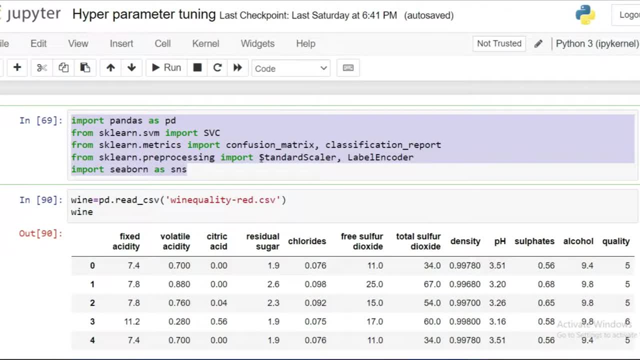 now to show your support. Okay, The first cell of the Jupyter Notebook. I imported some necessary libraries for my model development And in this experiment I'm going to develop support vector machine model And I will show you the model accuracy differences before and after implementing. 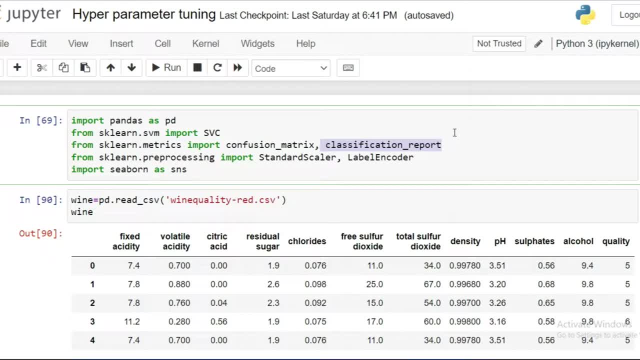 that parameter tuning- Okay. And for evaluating my machine learning model, I'm going to use classification tuning- Okay. And for evaluating my machine learning model, I'm going to use classification report matrix to know the accuracy differences at the end. So these are the requirements that are needed for my model development and hyperparameter tuning. 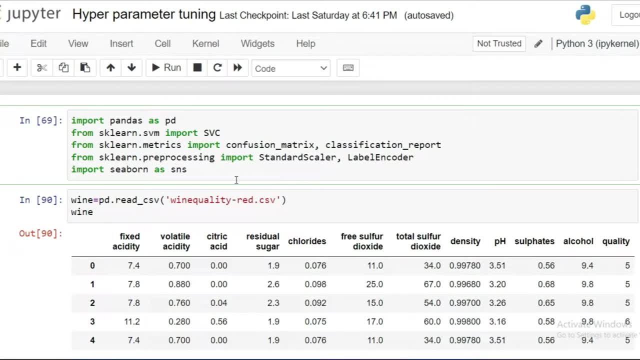 So let's start the data preparation part, And if you want to skip the data preparation part, you can skip by using timestamps. I will provide the timestamps for this video in description. Okay, So now look at the dataset. This dataset is not prepared, So we have to do some changes before. 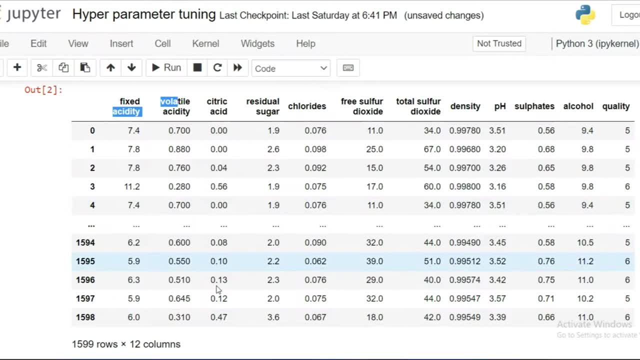 we implementing the SVC algorithm on this dataset. So what are the preparations we have to do? So first of all, let's look at the data set carefully. In this dataset there are 11 features are there, and quality column represents our target. So in the target column we have different types of 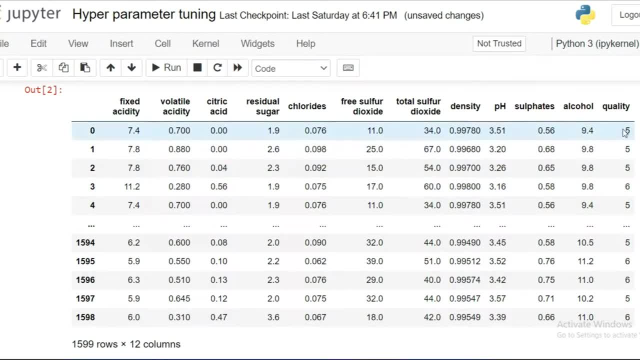 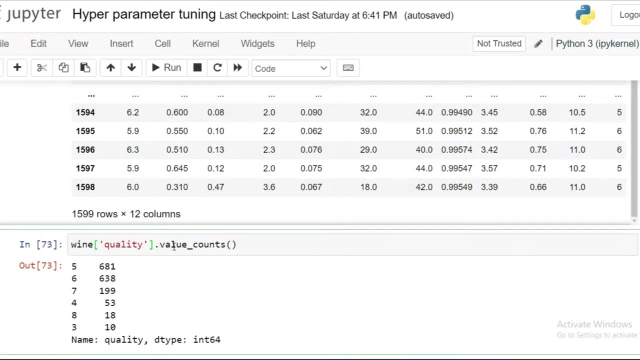 wine quality numbers are there And initially we don't know which quality of wine is good, So these are just numbers. Okay, So these are just numbers. that doesn't denote anything to us. So in the first step of data preparation, we are going to transform these six values. 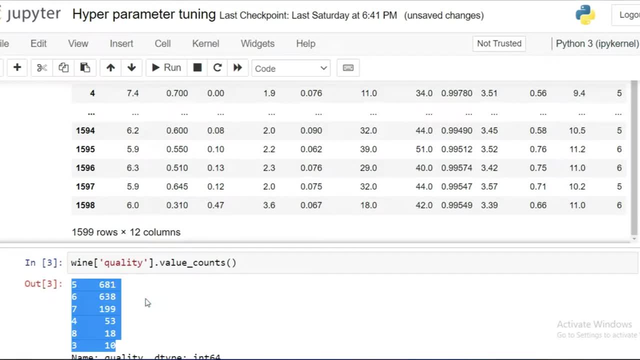 into two labels. So why we are going to form the two labels means I told we are going to use this data set. SVC is a classification algorithm, So our data set target should be in binary labels For transforming the data I'm going to use: cut function from pandas. So this is the first time. 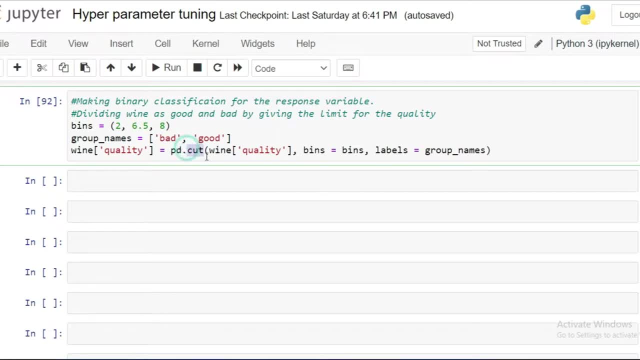 I'm using the cut function from pandas, So basically it will transform the numerical values into labels. Before running this cell I declared one variable called bins. So in this bin variable I set some data intervals, from two to eight, If the numbers are in the range. 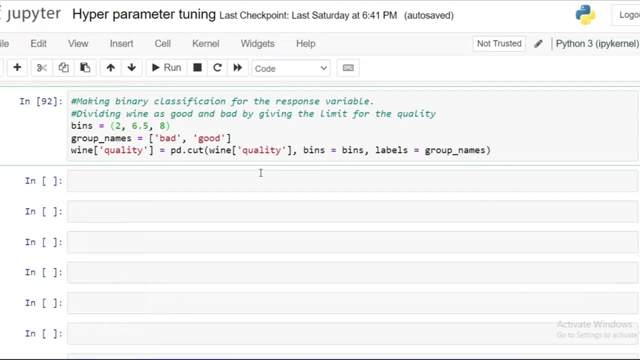 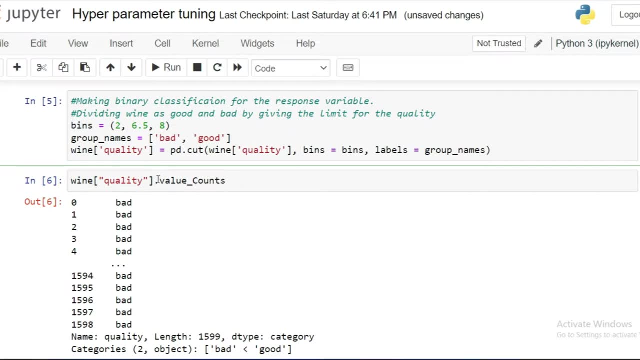 it will transform those numbers into the good and bad labels. Okay, so that's the concept about the cut function. Let's move to the next step. Now we get the labels like good or bad wine quality. Let's convert those two labels into. 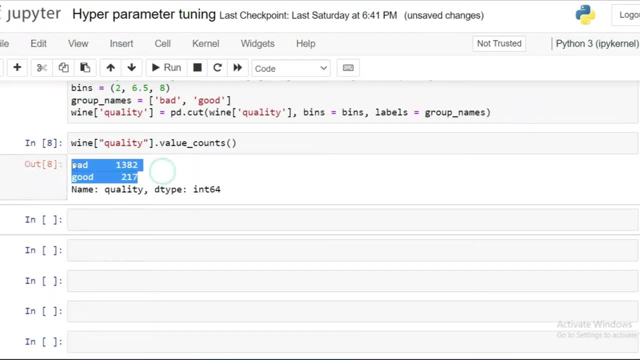 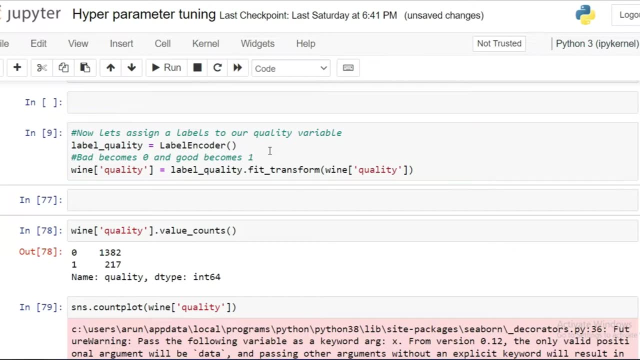 binary values. For converting the binary labels into binary numbers. Here I'm using label encoder function from scikit. learn to convert the labels into binary form. After transforming the labels, let's check how many bad and good values are classified in the data set, So you can see here. 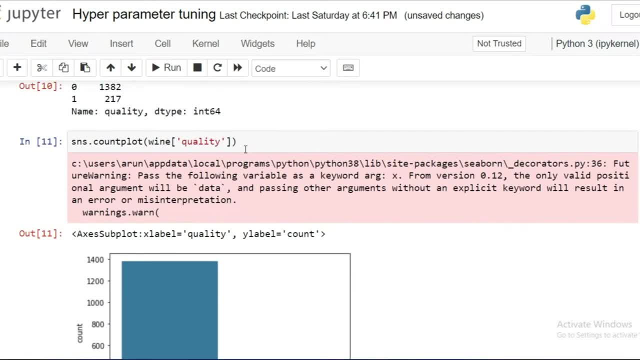 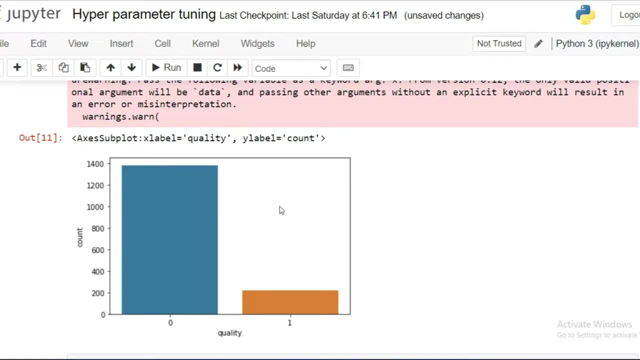 there are 1382 values are classified as zero and 217 values are classified as one. Here, zero represents the bad wine quality and one represents the good wine quality. Next I'm going to allocate feature, So in this cell I'm dropping the quality feature. 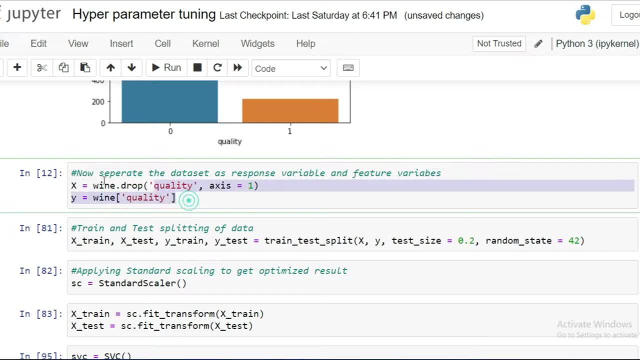 from the main data set In the X variable. it contains 11 features except the quality feature, because quality feature is our target, So I'm allocating a Y variable for the quality feature. Okay, so now our data set is ready. Let's move to the next step In the next step. 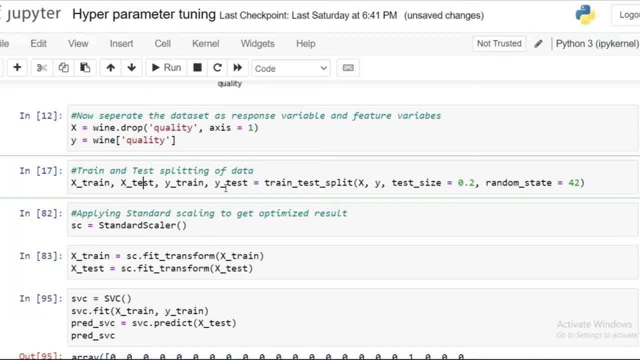 I'm splitting the data set into train and test. After splitting it, I'm going to scale. I'm scaling my values in the data set. So why I'm scaling? means to achieve the faster processing and optimize the results of my model. So it is one of the good practice in machine learning you should 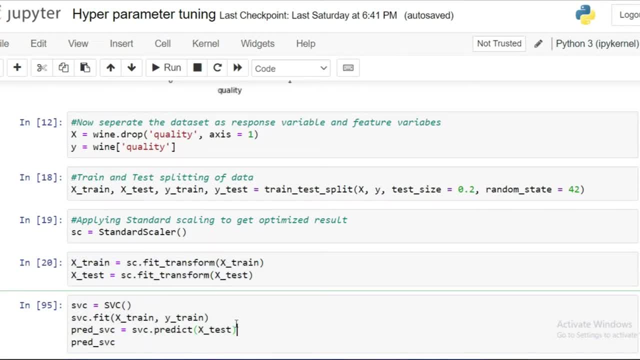 use the standard scale function, or min max scale function, to transform your data set values. It helps you to produce more optimization and stabilization to your model. Okay, after that, I'm training and testing my model with the SVC algorithm. So once I get the test values, 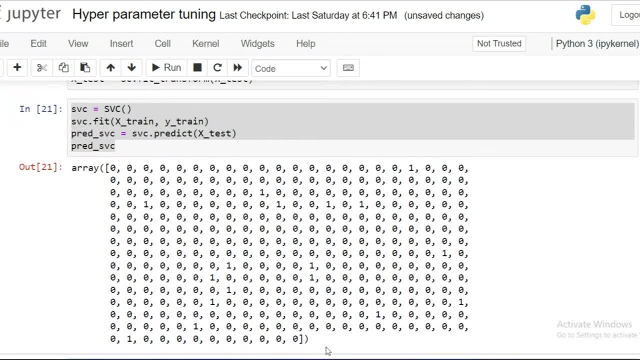 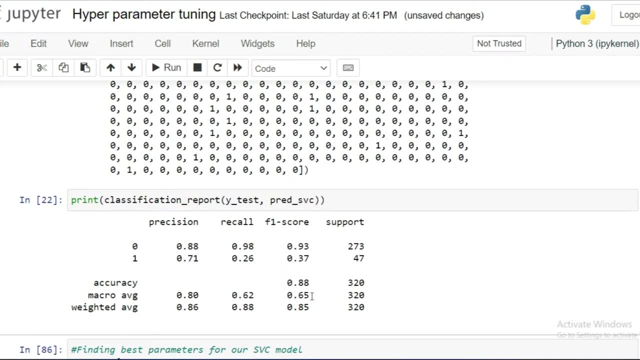 I'm going to generate a classification report against my model performances. So let's run the cell. So look at the classification report carefully. Here I got the accuracy of 88%. It is not that much bad. But this model trained with the default parameters of SVC. 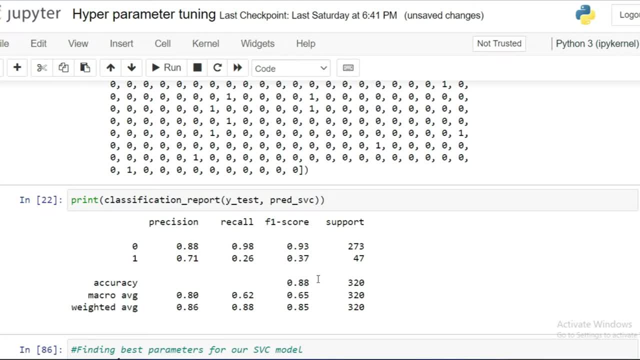 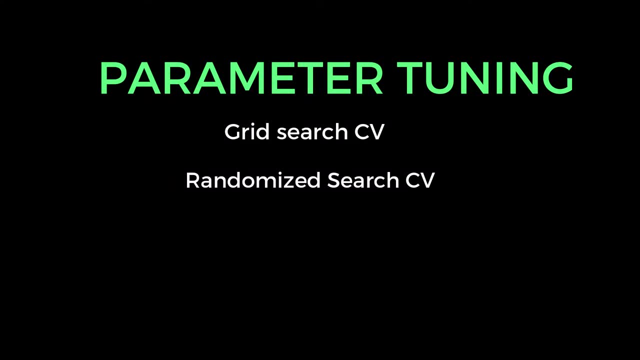 we don't get the best parameters for this data set. So for finding the best parameters, I'm going to use grid sets CV. If you're implementing parameter concept in your machine learning model, there are two popular methods are there in machine learning. One is grid set CV. 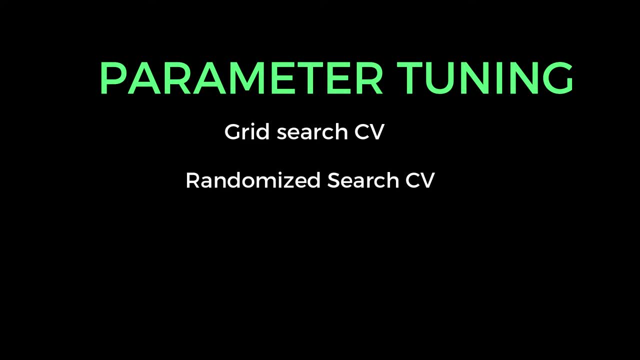 and another one is a randomized research CV. The difference between these two is, if you're implementing the grid set CV, we have to give some expected parameter range values. the grid set CV only implement that expected parameter values that you're given, But the randomized research CV